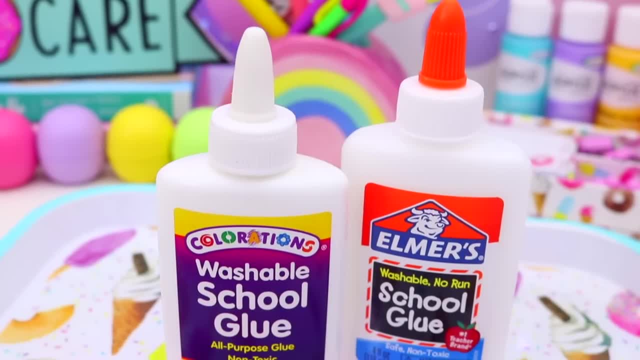 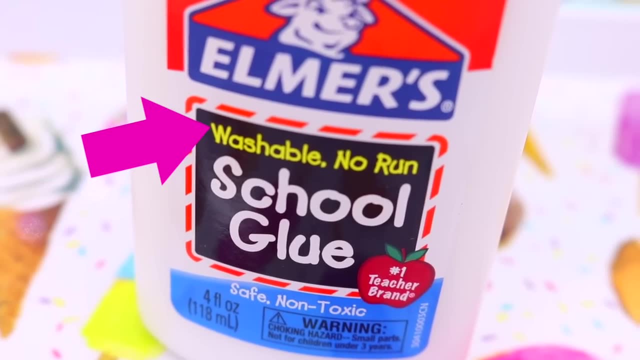 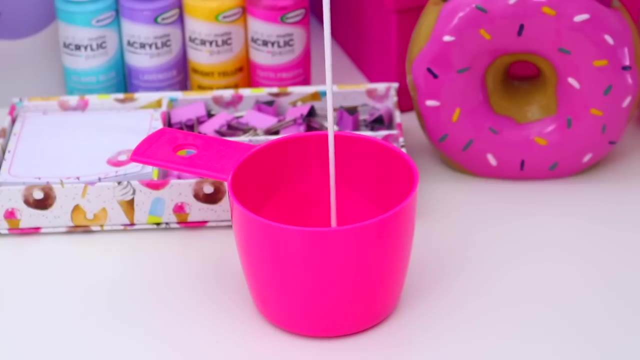 to need one cup of PVA glue or school glue, and what I found is glues that say washable tend to always work really well. so I always try and find a washable school glue and then it usually works. so that's just a little tip for you. So just take one cup of the glue. 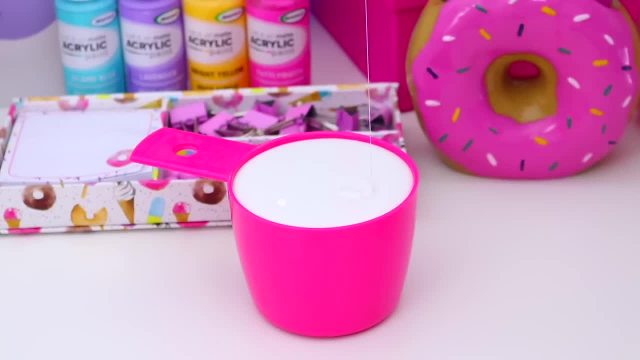 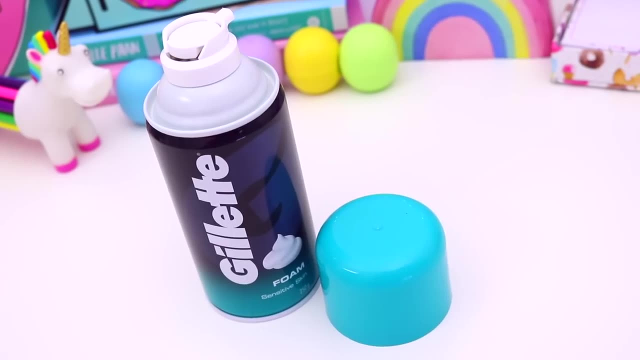 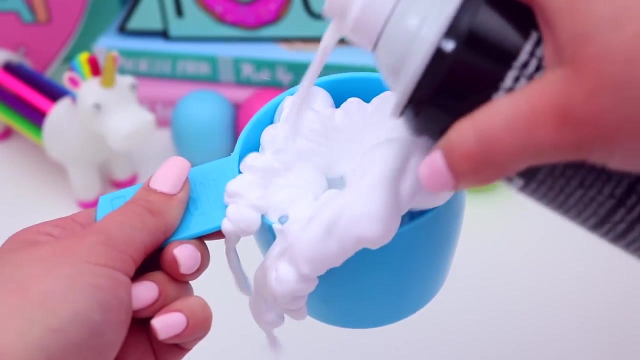 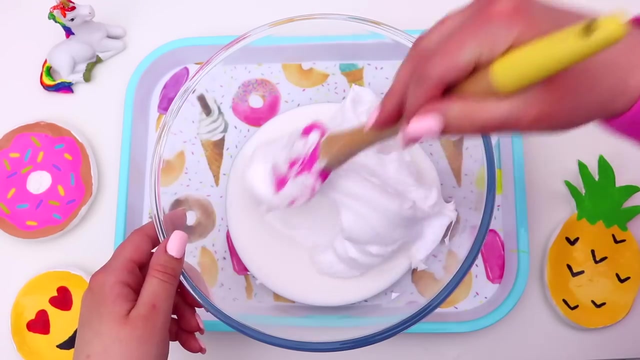 and add this to the bowl Now, because we are making a fluffy slime today. to give it that awesome fluffy and lightweight texture, you're going to need one cup of shaving foam, so just add this to the glue. and this is my favorite part about making fluffy slime, because it always looks like whipped cream. 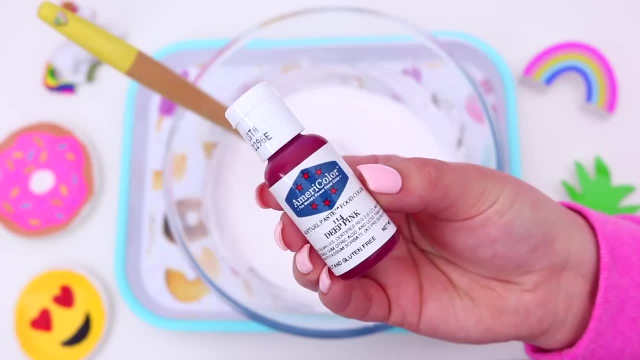 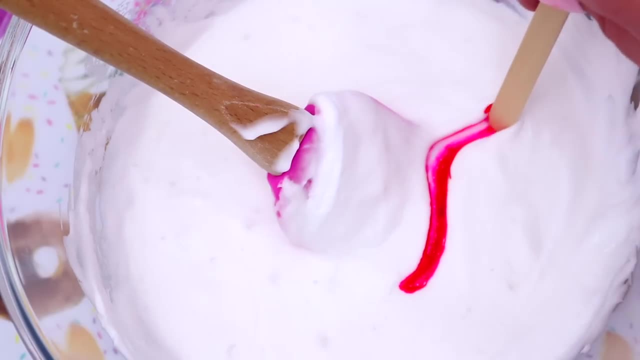 Now we need to give our slime some awesome color. so just take some food coloring and, because this is a cotton candy theme slime, Let's take some food coloring. Now I've brought a little bowl and our slime is all set, and I'm first going to be making a pastel pink slime and my favourite type of food colouring. 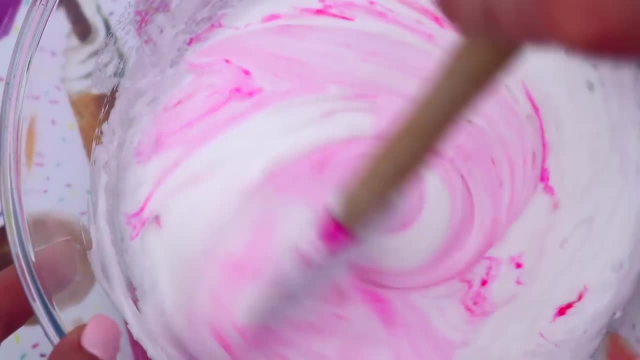 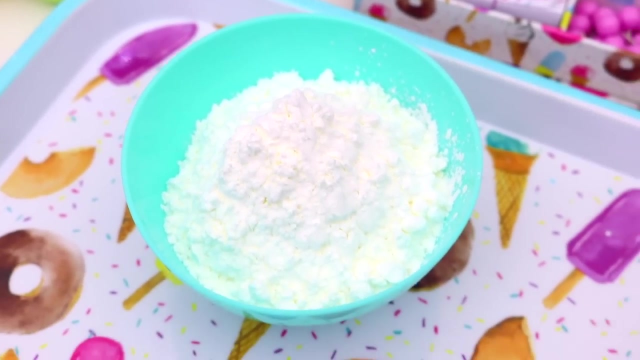 to use is gel food colouring, and I just add a little bit at a time because it's always easier to make it more vibrant, but if you add too much, it's kind of hard to fix it. So then you're going to need to take 1 tablespoon of cornstarch and add this to the glue mixture. 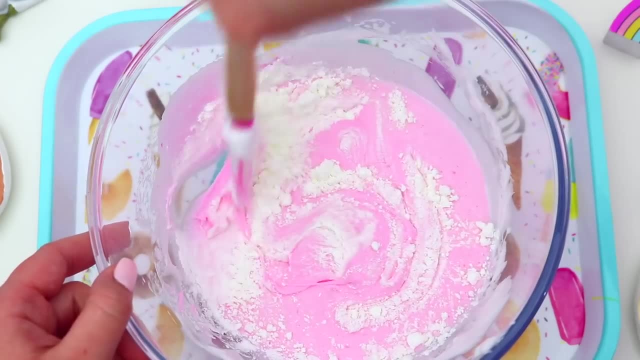 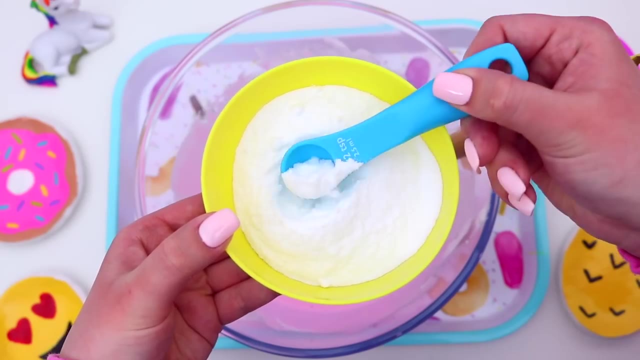 and this is just going to give our fluffy slime some structure. So then just mix in the cornstarch, and then we're going to need half a teaspoon of baking soda. so just go ahead and add this to the glue mixture as well, and we need to add this. 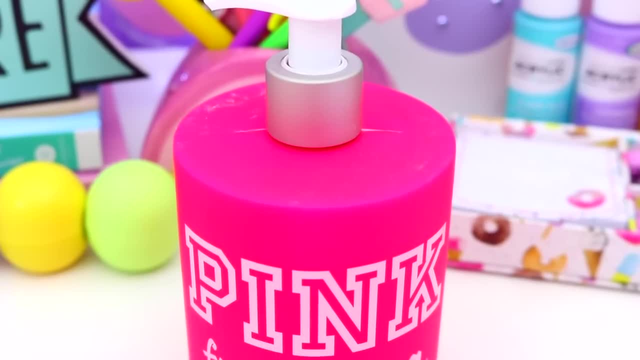 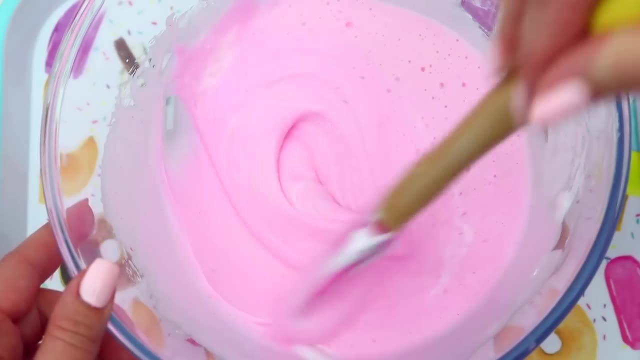 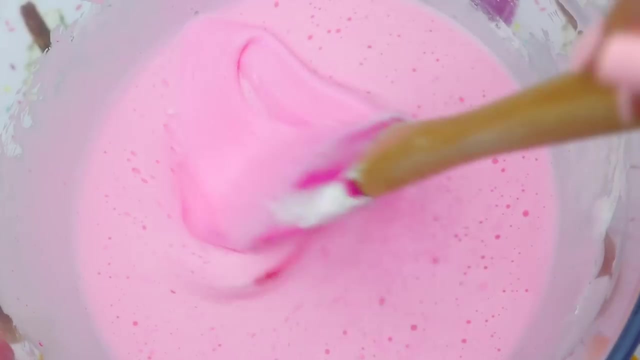 otherwise our contact solution, which is our activator, won't work. So now this is an optional step, but I always love to add a little bit of hand lotion or body lotion, and this just makes the slime super, super stretchy. Now this step is also optional, but to give it that full cotton candy effect, I added some. 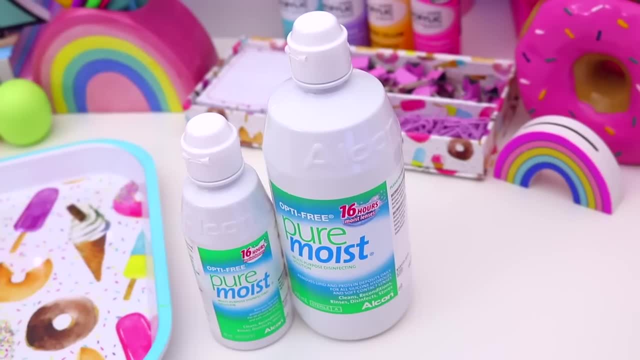 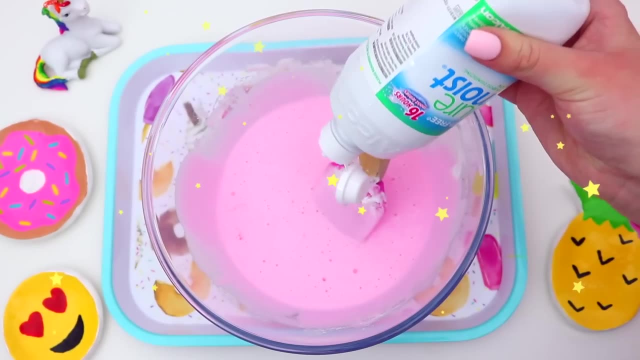 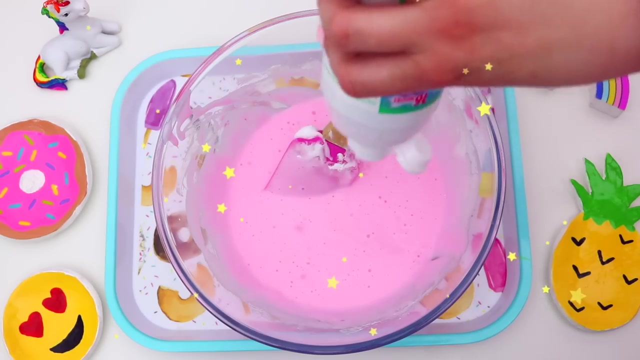 cotton candy flavouring and this made it smell so amazing. So now for our activator. We are going to be using our cotton candy flavouring. As you can see from the ingredients, it contains something called boric acid, which is similar to borax. so this is going to be our activator, and I love using contact solution just because. 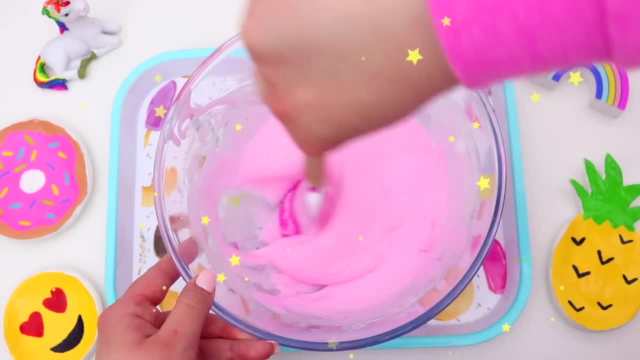 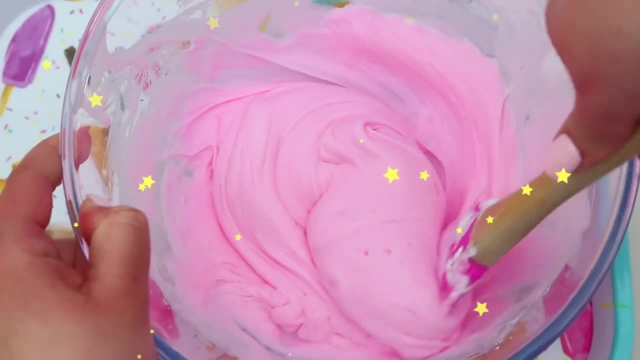 it's such a safer method and I just find it so much easier to use. So all you need to do is add a little bit of contact solution at a time. You just want to take this super slowly and make sure that you mix in all the contact. 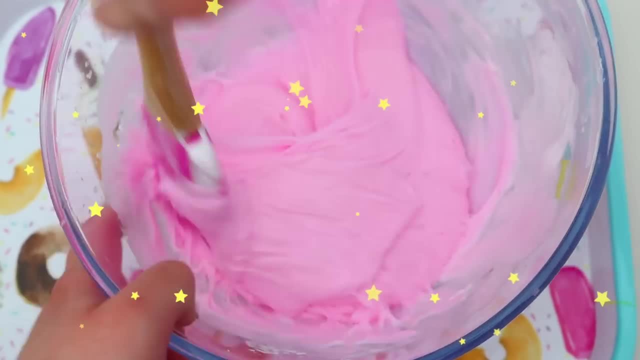 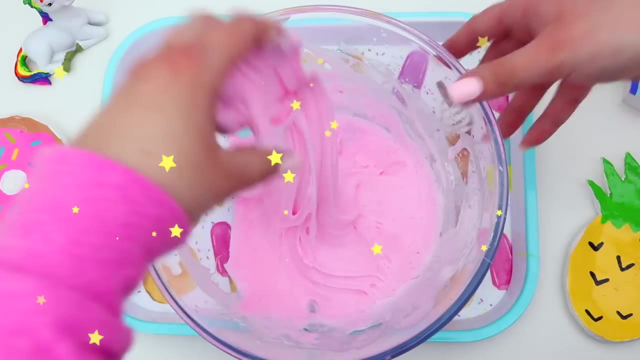 solution before adding more. Now you'll see your slime start to form And if it's still sticky, just keep on adding a little bit of contact solution at a time, and sometimes I find it easier just to go in with my hands and start mixing it just. 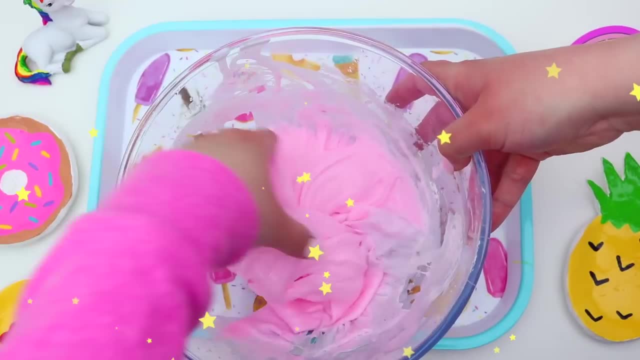 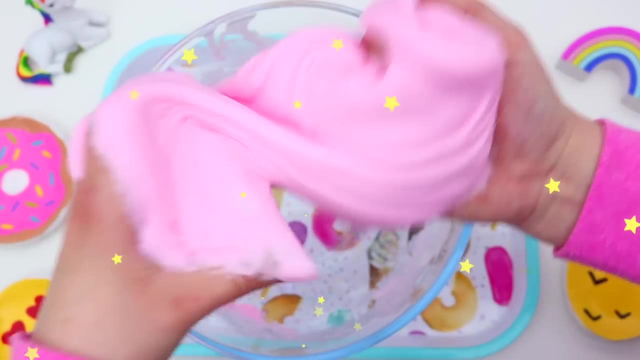 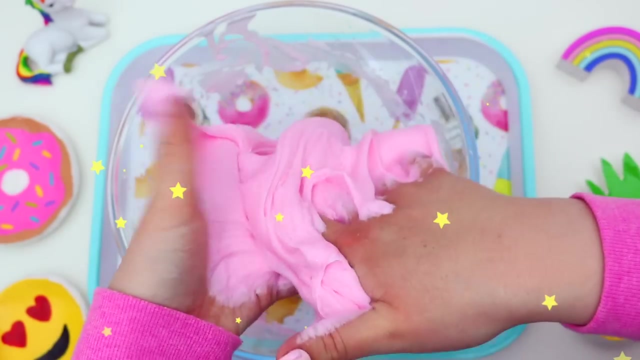 to see how it's feeling and, as you can see here, it's still way too sticky. so I'm just adding a little bit more contact solution and then working that in as well. So again, the slime here is way too sticky. You can see that it's still sticking to my hands and this is just not fun to play with. 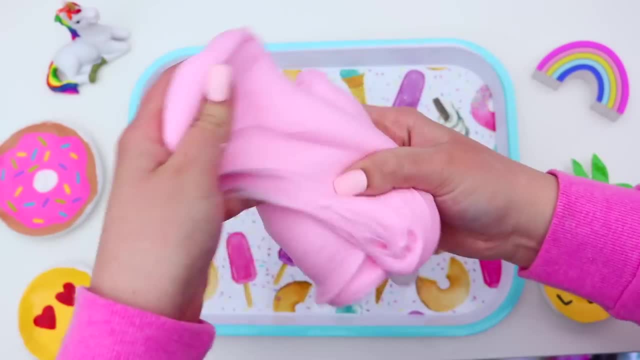 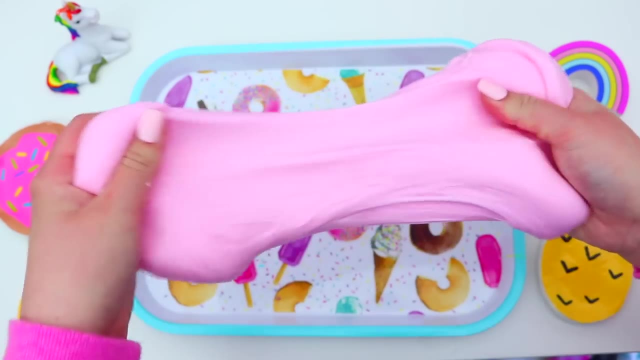 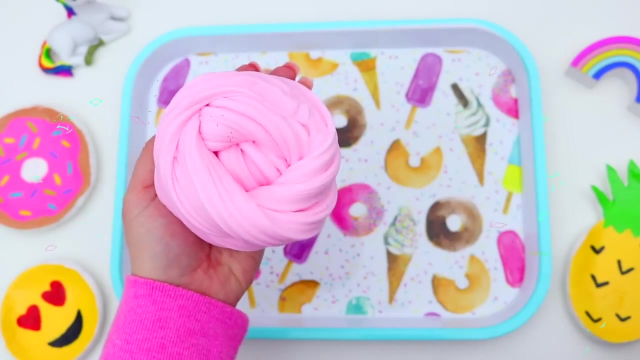 So I added a touch more contact solution and then after this, it was perfect and I had the most amazing fluffy slime, which also felt so incredible. I am obsessed with this color and the scent and this is just like the perfect slime and, yeah, I just love this slime so much. 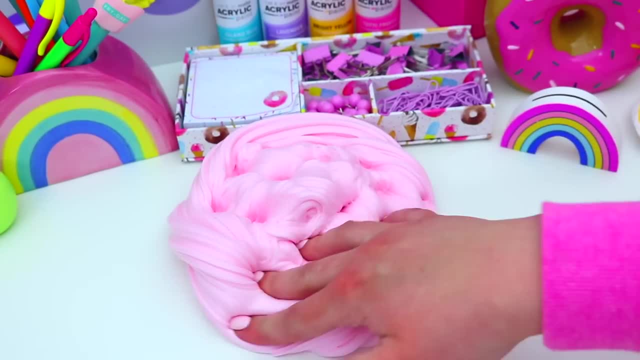 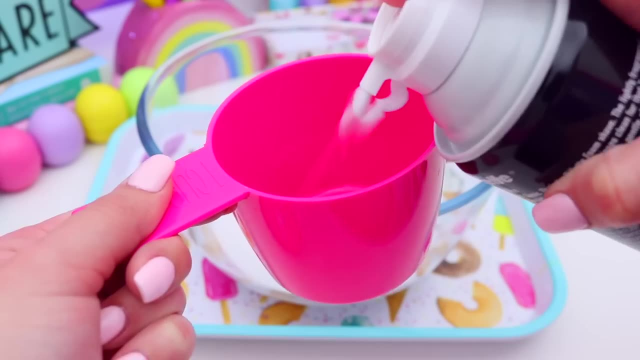 It's so pretty and it kind of reminds me of like a giant marshmallow. I don't know why, but seriously it is the most fun slime ever. So I decided that this cotton candy slime would look so much better if it was mixed with a cotton candy slime. 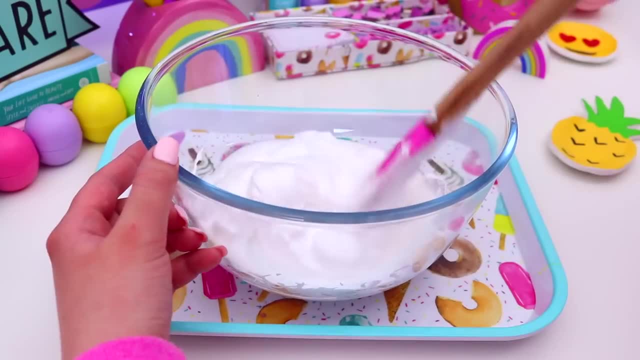 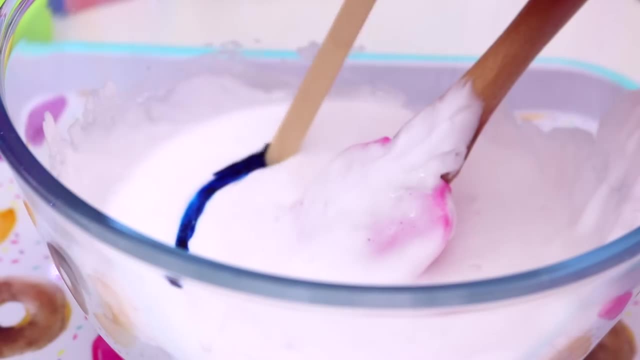 So I added a touch more contact solution and then after this it was perfect and I had the most amazing fluffy slime. So I'm just going ahead and following all the same steps with the cup of glue and the shaving foam and then with the food coloring, but this one is going to be a really pretty. 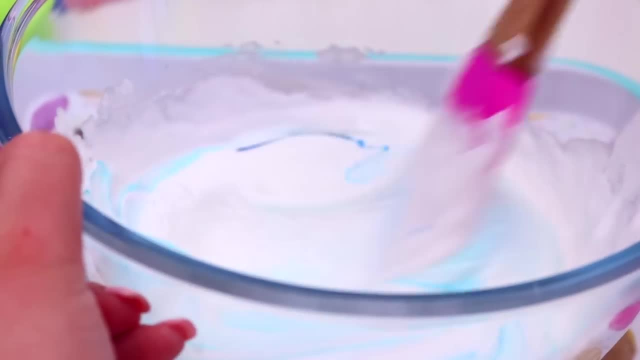 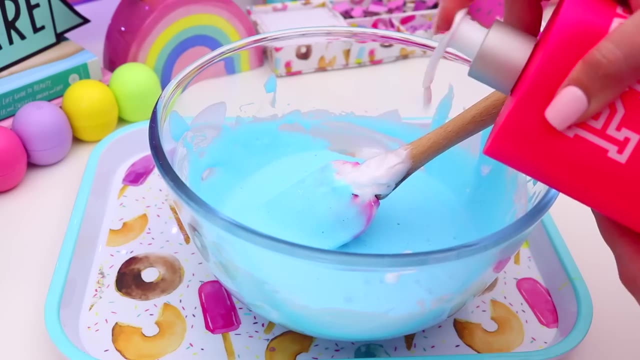 light blue color and, as you can see, I like to add my food coloring to like a popsicle stick or like a spoon and then add it to the glue mixture because I don't want to accidentally add too much and then have like a dark blue slime. 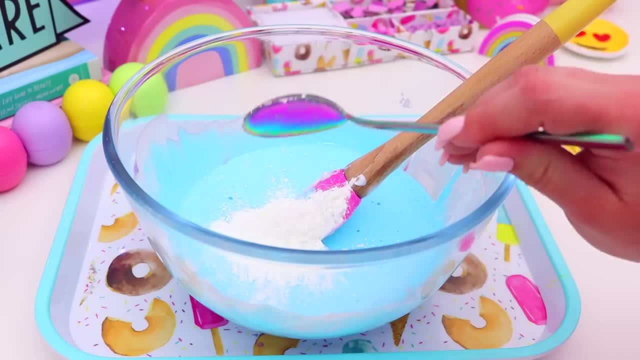 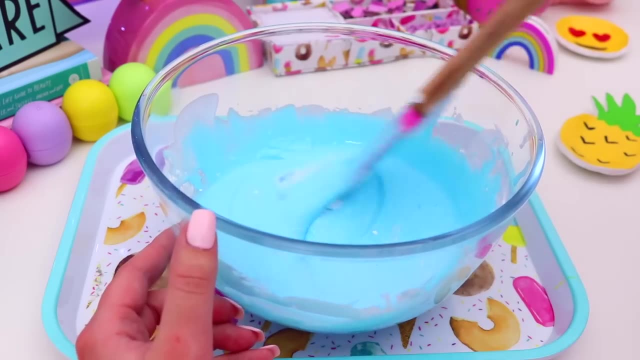 So I just like to add a little bit at a time, And then I'm just adding some body lotion, the corn starch and then the baking soda and mixing this all together and, as you can see, the slime is the prettiest blue color. 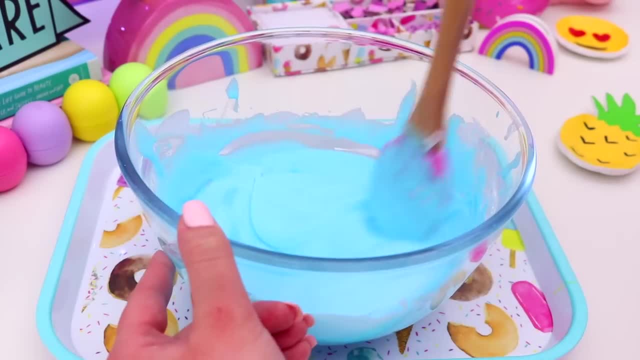 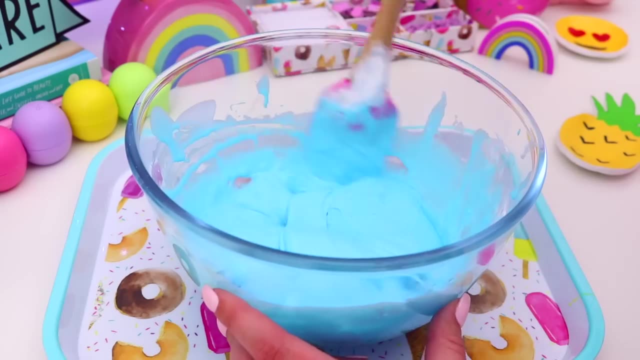 It totally reminds me of like the sky. so here I'm just adding some more of that cotton candy flavoring, because you can't have cotton candy slime without an amazing cotton candy scent. So now it's time for the activator, which is the contact solution. and again, following all